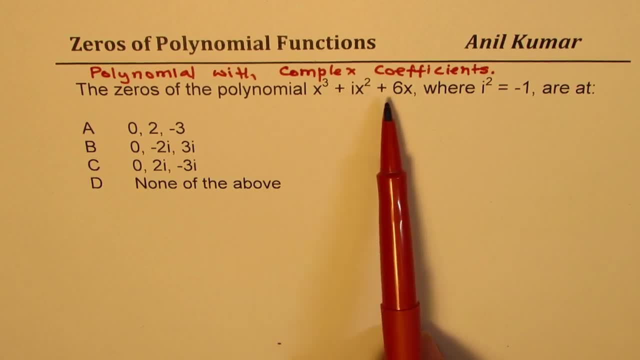 of a polynomial x cube plus i, x square plus 6 x, where i square is equal to minus 1, are at 0, 2, minus 3,, 0, minus 2i, 3i, 0, 2i minus 3i or none of the above. You can always. 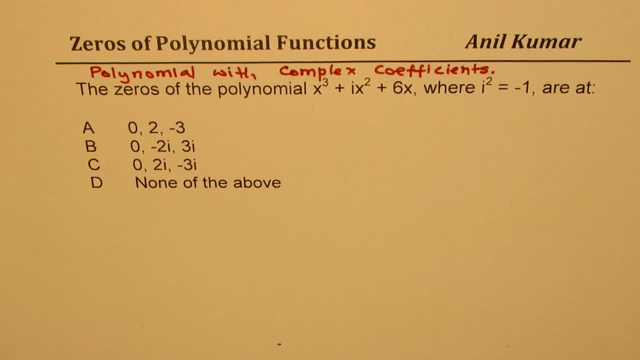 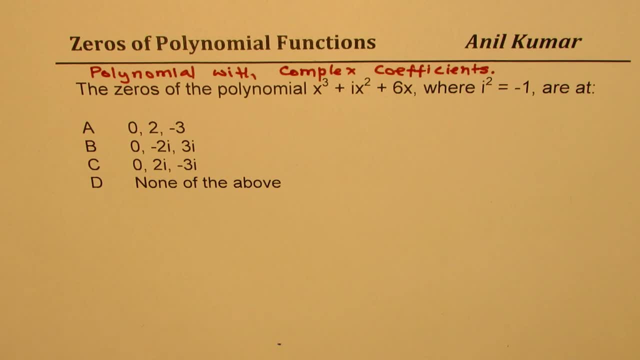 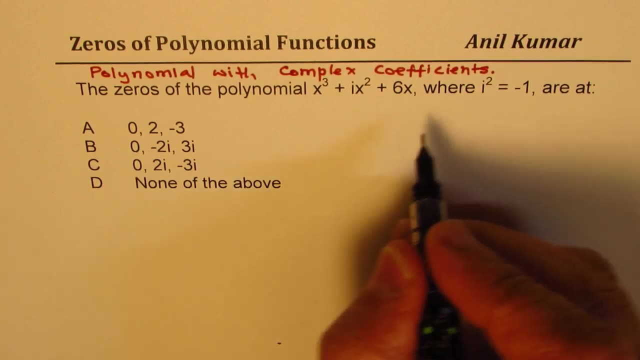 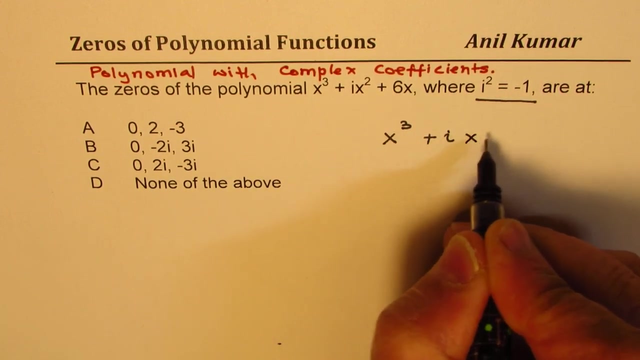 extend the techniques learned on factoring and see how they can be applied with complex coefficients. As you know, i square is minus 1.. So we are given x, cube plus i, x square plus 6, x as our polynomial with complex coefficients. So we have a polynomial with complex coefficients. 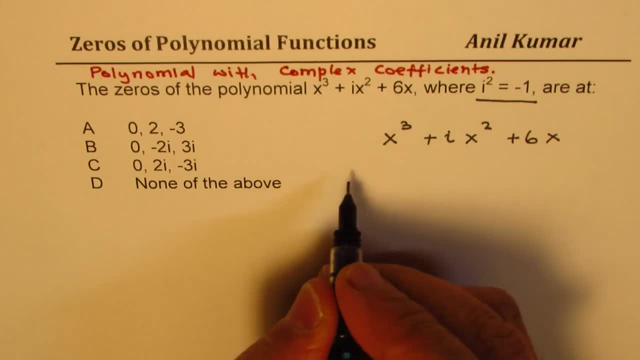 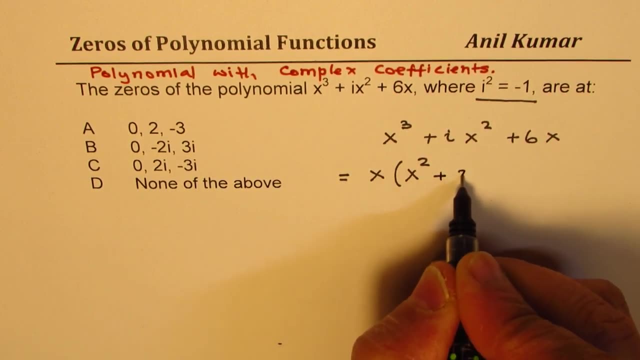 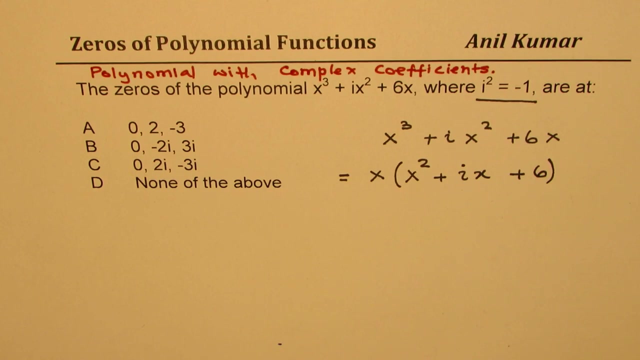 So we have a polynomial with complex coefficients. So we have a polynomial with complex coefficients- i Now we could actually factor x, So we get a quadratic trinomial: x square plus i, x plus 6.. The difference between this and what you normally use is that we have a coefficient which is: 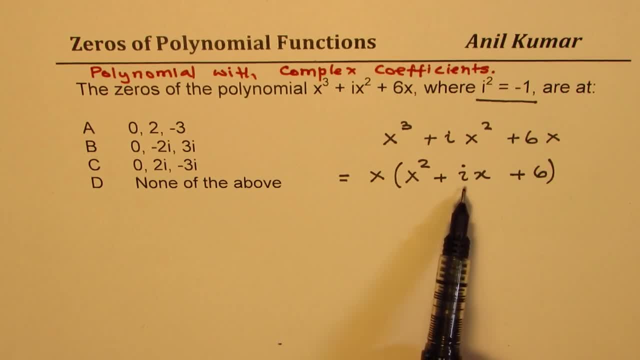 complex. So it is not a real number, It is a complex number. Now, how do you factor this using the factoring techniques? We know that we have a complex number, So we have a complex number. So we have a complex number. Now, how do we factor this using the factoring techniques? 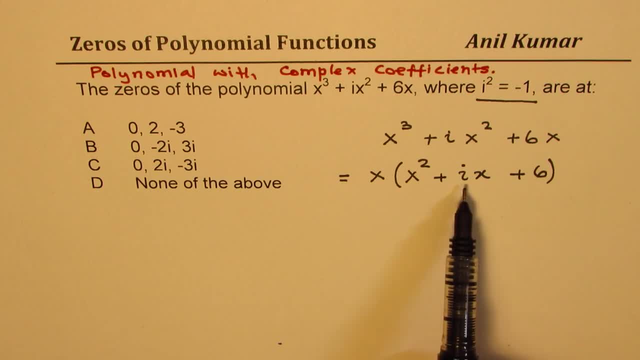 So product of 6, and we are looking for sum of plus i. Now how do I get that part? Now, this could be resolved if I write or change this equation in this fashion: i x. So instead of plus 6, let me write here as minus of minus 6.. So I have added this step to make my 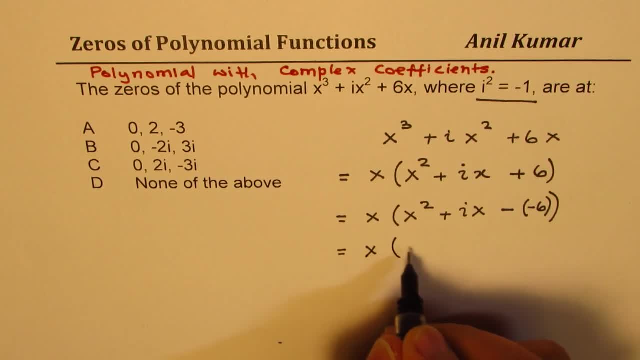 point clear, and that is to say, what I am going to do now is I will write the trinomial i square plus, i x minus. now minus could be written as i square right. so so i'm making this very important change here. i'm writing this as i square 6. do you see that part? 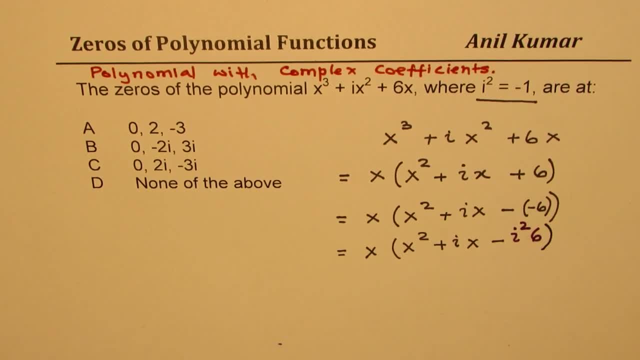 perfect. now, after doing this, we can look into sum and product. so we are looking for now a product which is i square 6 and we are looking for a sum which is i- x rather minus i square 6. do you see this part right? so i hope this is absolutely clear. the technique used to factor: 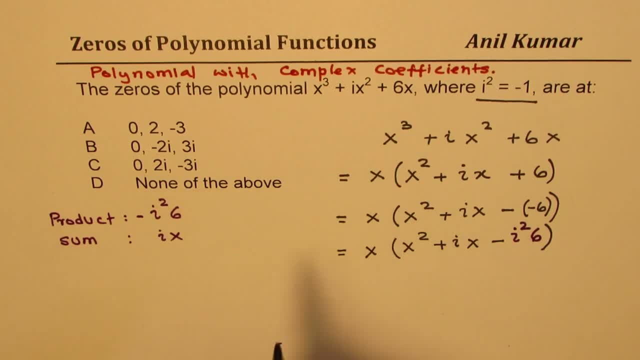 a trinomial with complex coefficients, right? so when you enter the domain of complex numbers, there could be some questions like this. so now you can see that i square 6 is a product which is i square 6, and we are looking for a sum which is i x rather minus i square 6. do you see this part right? so i hope this is absolutely clear. 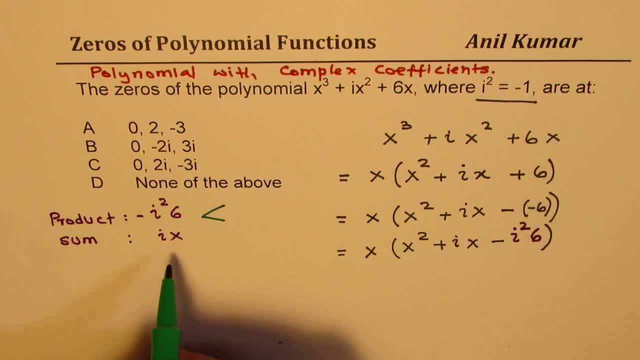 since we need this as positive, we are looking for a positive, bigger number: three and two. so we have three i and minus two i. so when you add them up, you do get i, so that becomes the key. so using these numbers, we could now factor this as x times x plus three i. 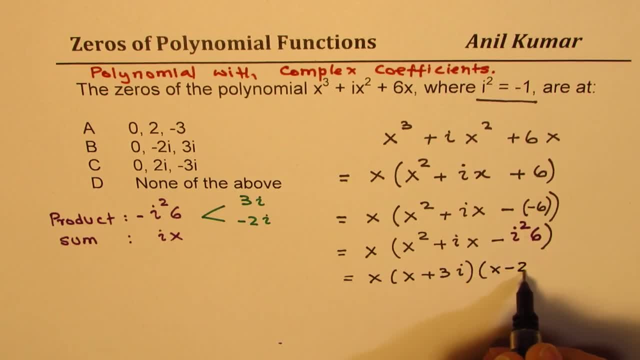 times x minus two. i does make sense, right? so that is how it could be factored. you can always verify by expanding and checking whether it really works or not, right? you could do that now, once we have factored, now we know the zeros. so one zero is, of course. 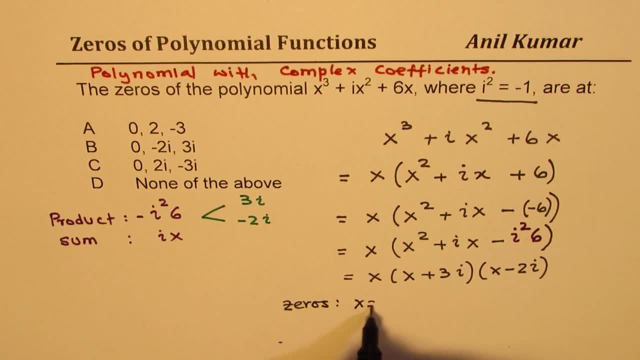 at x equals to zero. the other one here will be at minus three, i right. so this is at x equals to minus three. i and the third one is at x, equals to two. i. is that clear to you? so the option c is the correct option. perfect, so that is how you could actually factor. 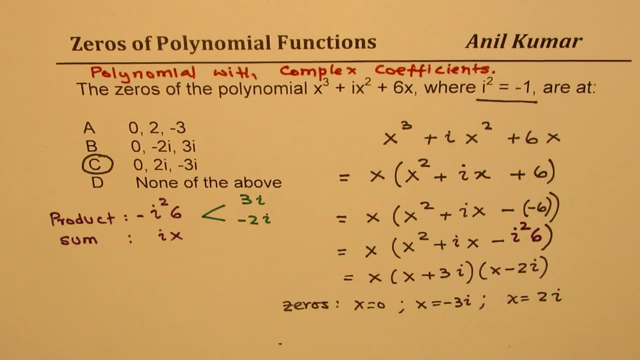 polynomials with complex coefficients, so we are working with complex numbers. so in this domain, as you know, i square is minus one. so the idea here is that if you have i as a coefficient of any of these complex terms in a polynomial, in that case the constant. 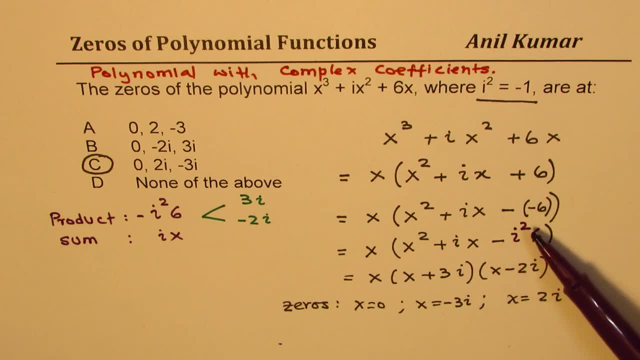 term is going to be i square minus one. so that is how you could actually factor polynomials with this term could be replaced by minus i square right. so because i square is minus one and minus and minus one will be plus one, correct? that's the whole idea. so that is how we could.